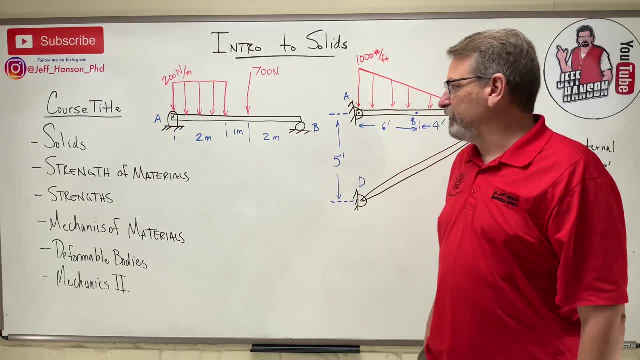 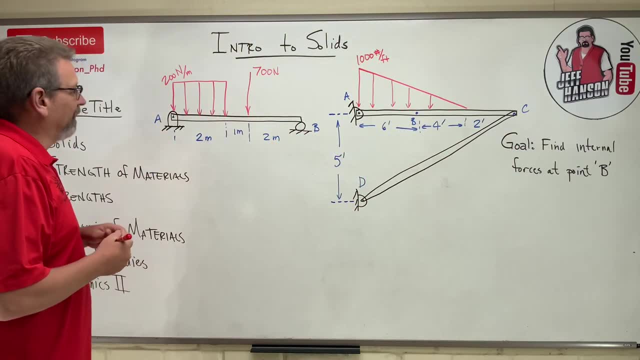 with fine-globalization, So you all know what that means. right For a question like this, right? This is just a little simple truss problem, right So, but not a truss, a beam, But what you have to do, right, You've got. 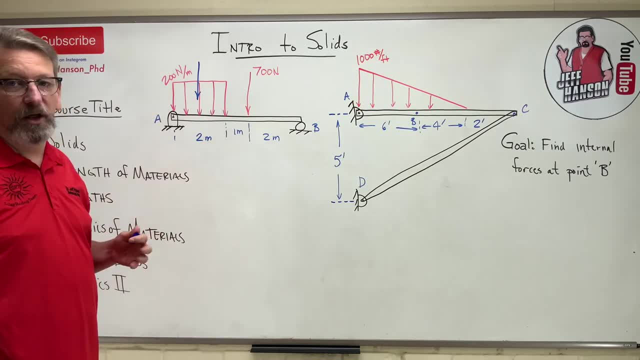 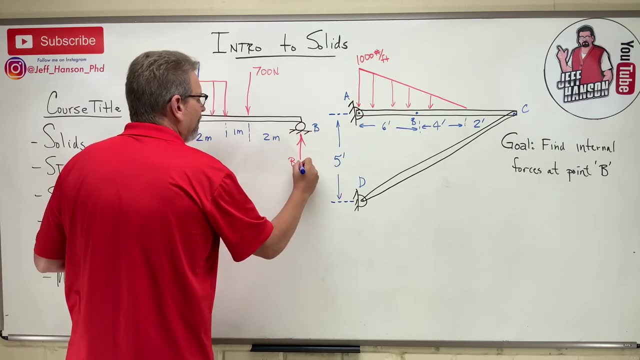 to be able to convert a distributed load into a concentrated load, You've got to remember the reactions at the support. So you would have a BY and you would have over here an AY and an AX right And you should be able to. 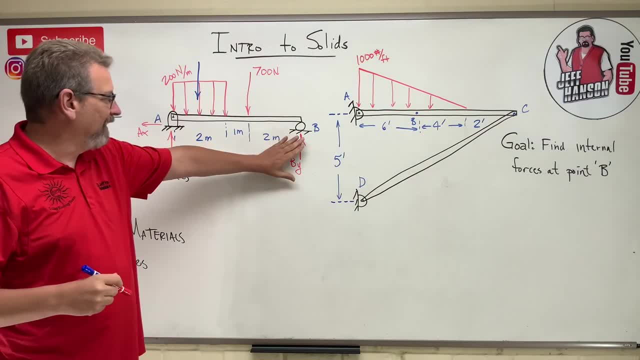 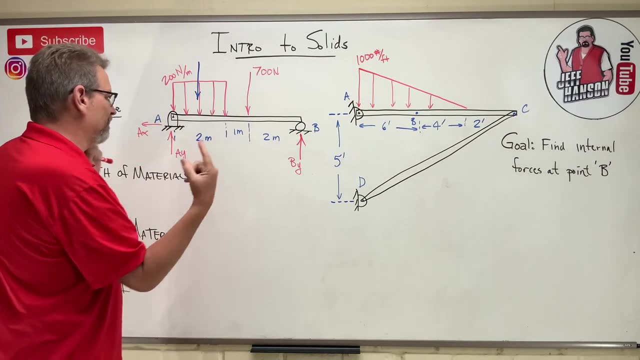 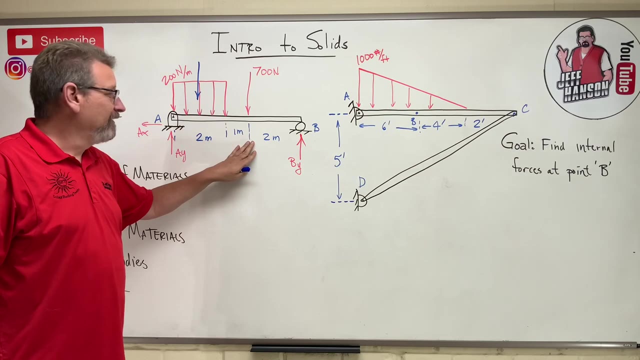 remember how to come up with those. I've got to take the moment at A to find BY, Then come back and sum the force in the Y to find AY. The first step in every solids problem is going to be just like that, okay. So if you're weak at statics or you just barely pass statics, you know. 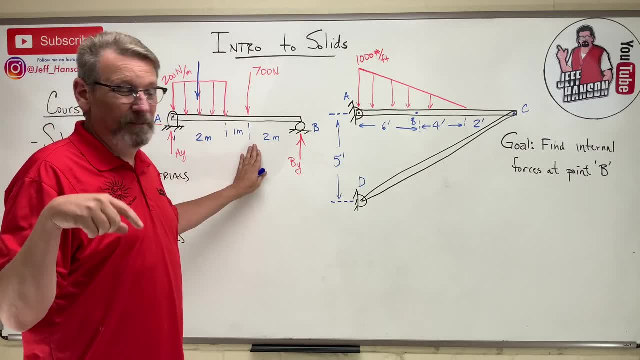 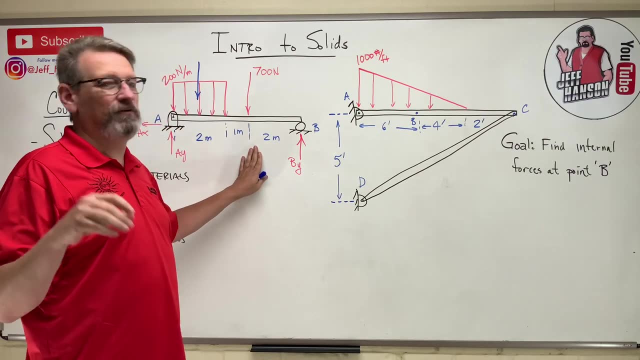 it would pay you dividends to go back to my statics series on YouTube and review those videos, because it will get you a better foundation in statics. okay, So, if you just kind of go through those, Because, man, if you're going to struggle on the global equilibrium portion of this, 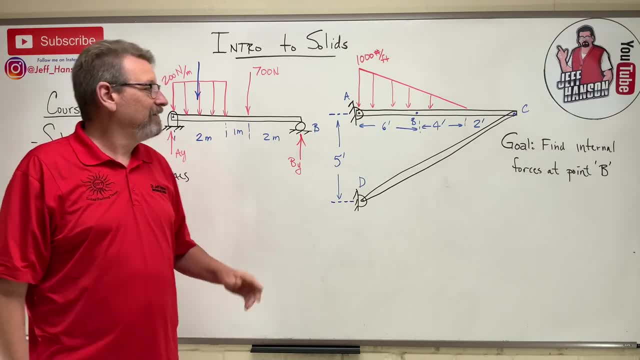 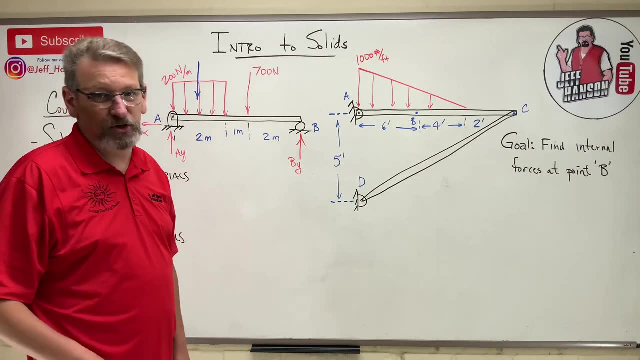 then this class is going to punch you in the face. okay, So you know something like finding the reactions of global stuff here. I expect that that should take my students about two minutes to do. You ought to be like bam- I know how to do that from the other class. Wham, I got it you. 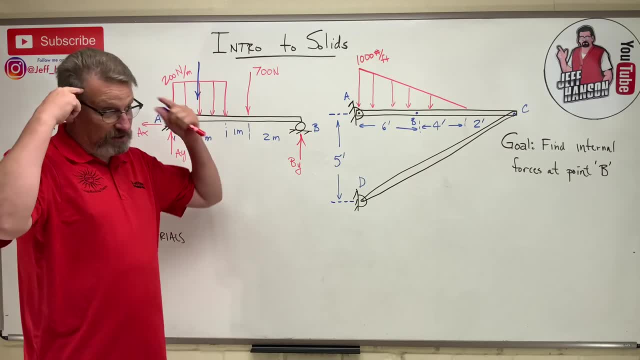 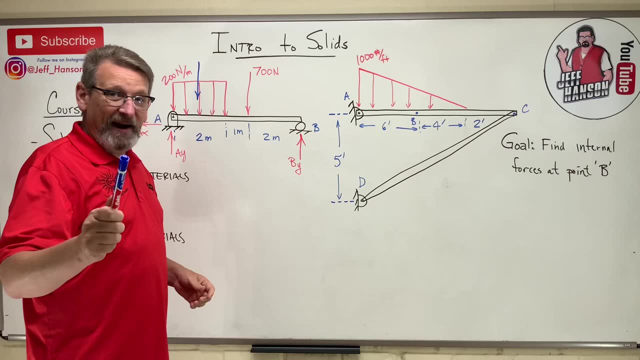 know, And if you're struggling with this, still I don't remember which is cosine and which is sine. This class is fixing to kick your hiney, okay, So get prepared, Okay, And so you know. one of the things I want to do is start off with something simple here. 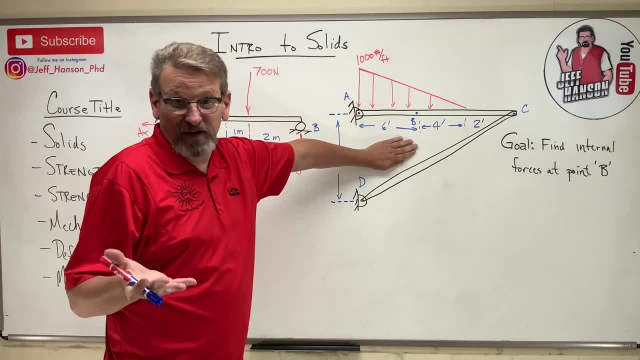 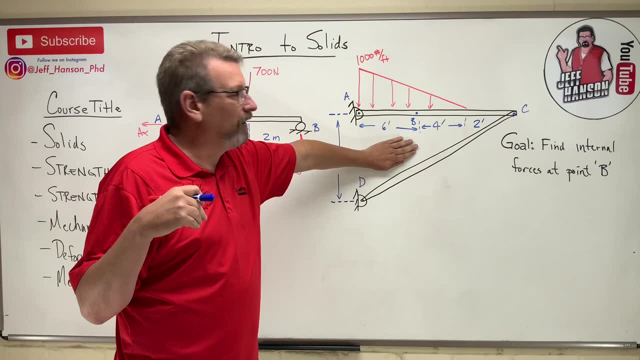 The very first problems in the solids book are nothing more than a review of classes from statics. So I thought it would be best let's just start off with one little statics problem. Let's see if we remember how to do this And we'll work through something like this: Find the internal. 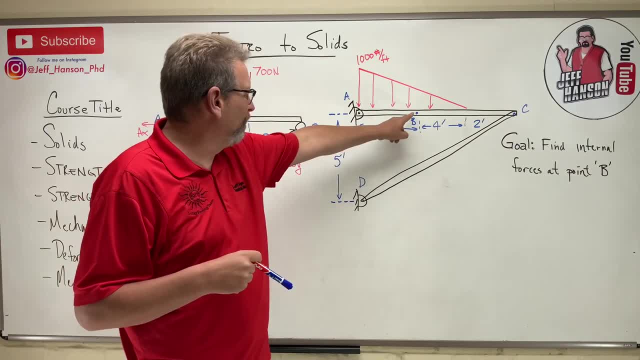 forces at point B. Here's point B right there. So let's see if we remember how to do this right quick And this would be a good review. So let's start off with one little statics problem. Let's see if we remember how to do this right quick, And this would be a good review And this would be a good. 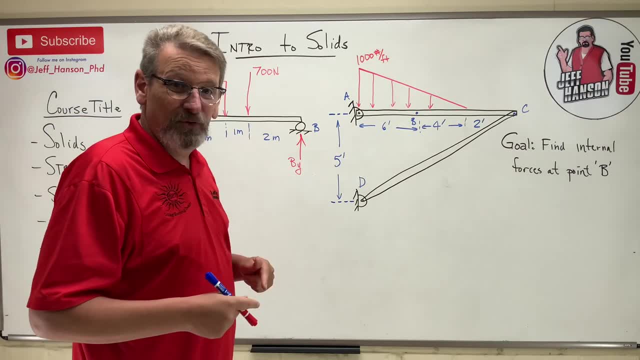 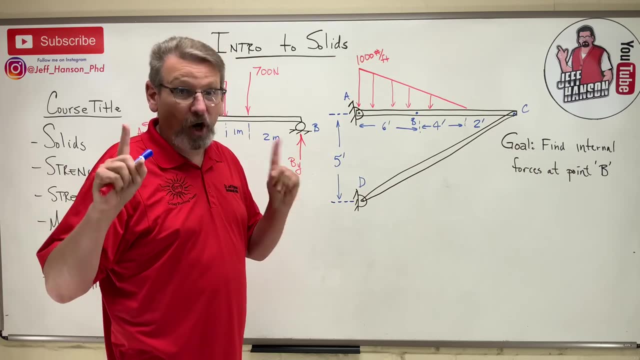 review And then the next video. we're going to start off with some new things Now: statics, all the equations. we just made them up as we went along right In solids. there are a lot of equations, There's a lot of equations, And so it's important that you stay up with this. It is 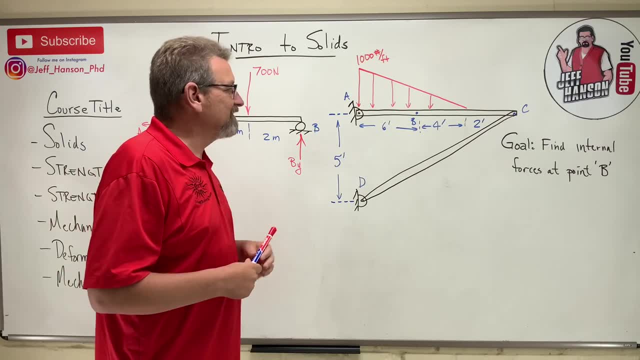 a harder class. I promise you that. So let's see if we can do this. I want to erase some of this. give us some room and let's see if we can work this problem out here. All right, y'all hadn't. 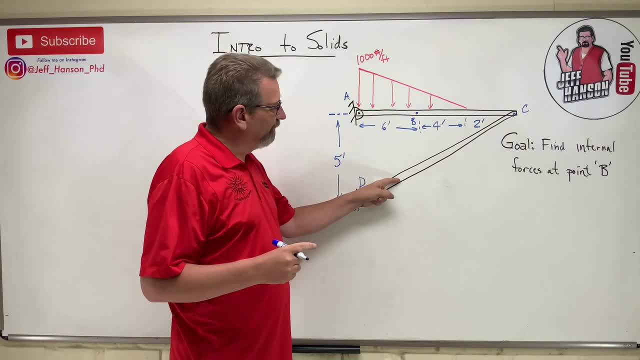 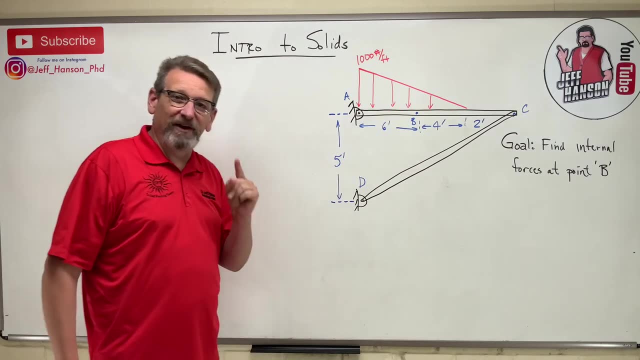 gotten soft on me, have you? Do you remember what this guy here is? What is that guy? That's a two-force member. pin connected at both ends. no forces in the middle. two-force member. I remember those guys okay. 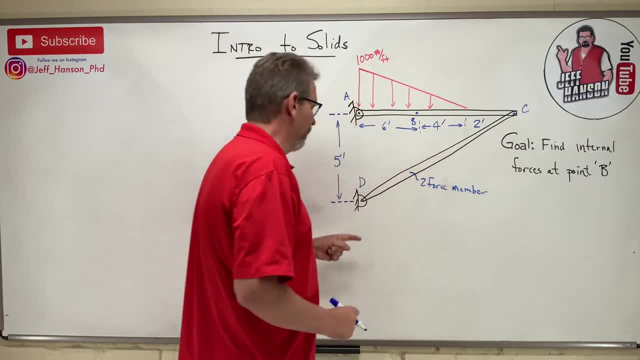 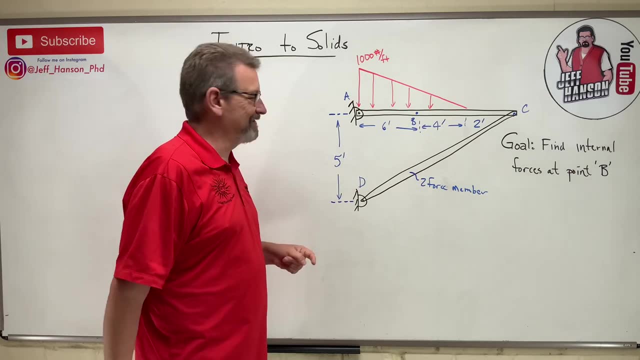 You got to remember all of this stuff, right? Because Johnny Weak Sauce, he says: hey man, pin connection there, pin connection there. that's four unknowns. I can't solve this. But we're like: no, Johnny Weak Sauce, that's not two unknowns, that's one unknown because a two-force member. 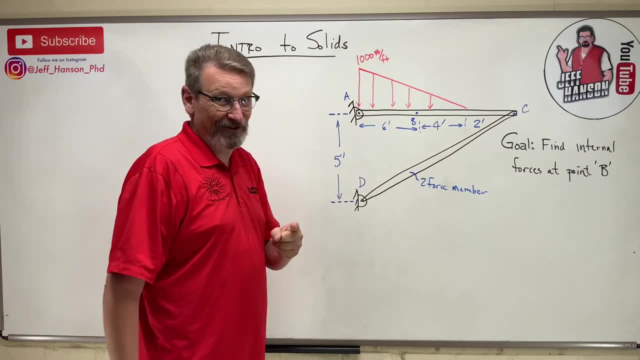 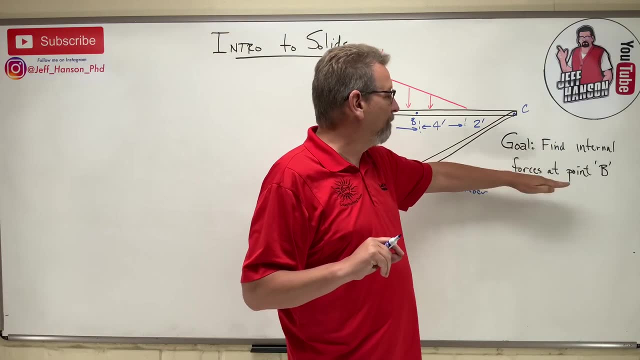 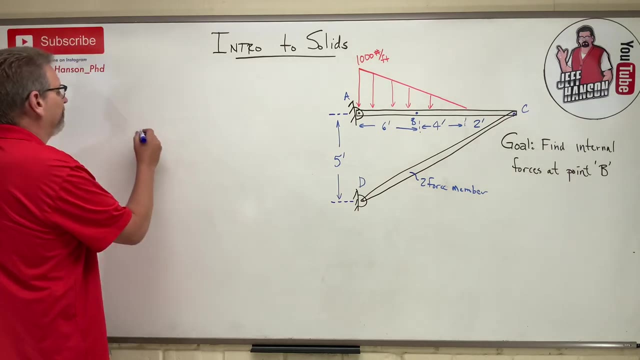 takes you from two unknowns to one unknown. I learned that in Dr Hansel's statics class. Yo, Okay, step one to solve this problem, to find internal forces at point B- is to solve for global equilibrium, right? So let's draw a free buddy diagram, Okay? so here's that beam. 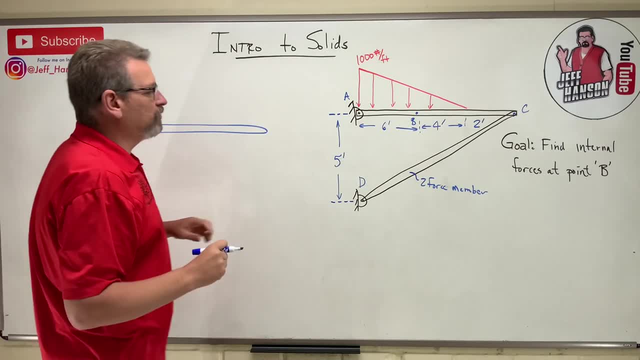 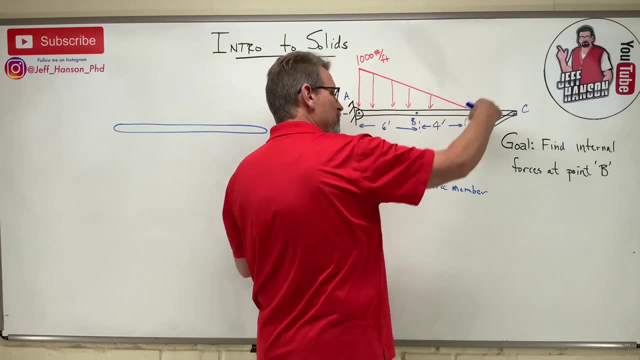 the top beam up there and the two-force member. we'll call him FDC, right? Do you think he's in tension or compression? This whole thing is pulling down, so he's squeezing him. So what's his reaction to me? 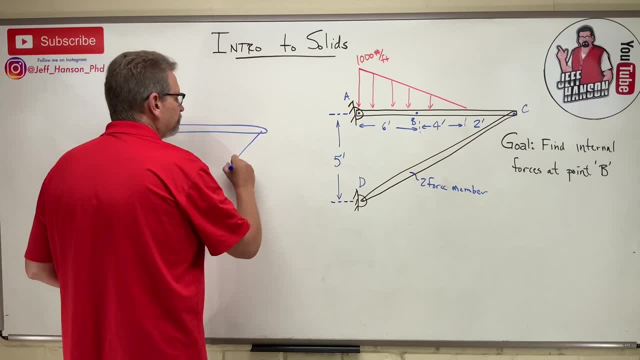 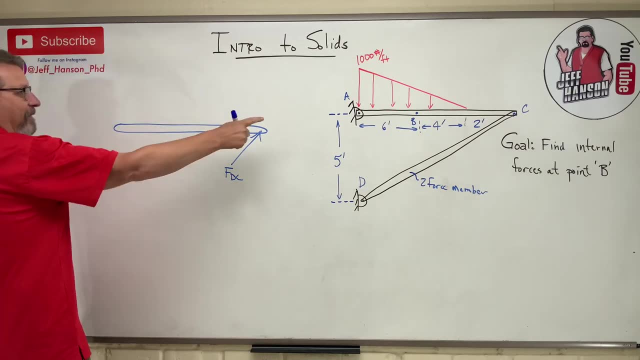 Push back right. So here he is, FDC pushing back on me, okay, And then over here, at point A, that's a pin connection. So you've got an AY and an AX. And then up here, what do you have? Well, you have a distributed 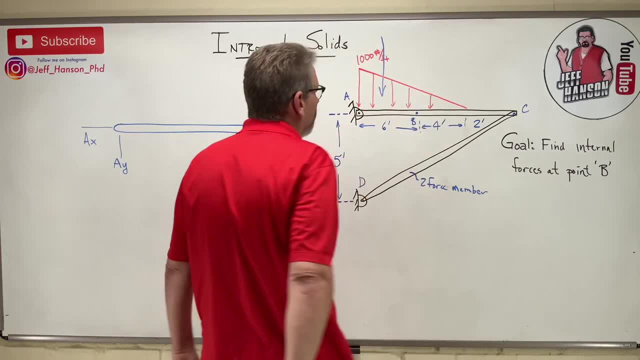 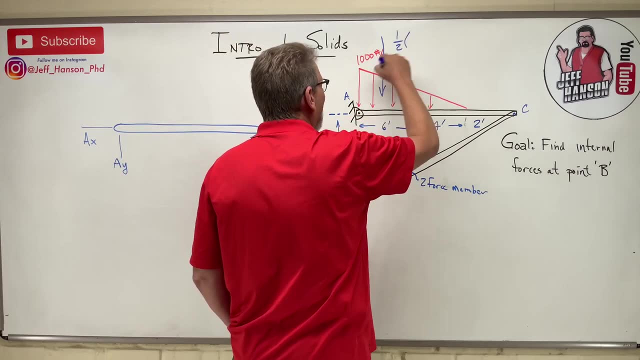 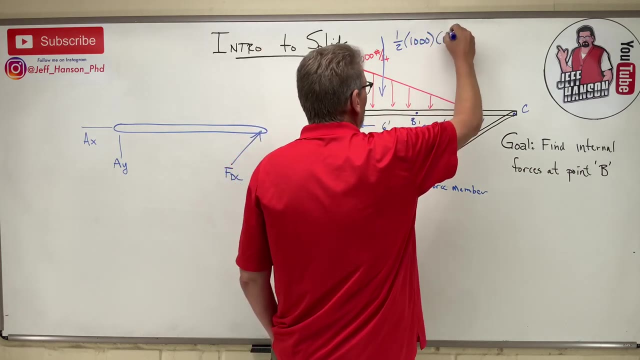 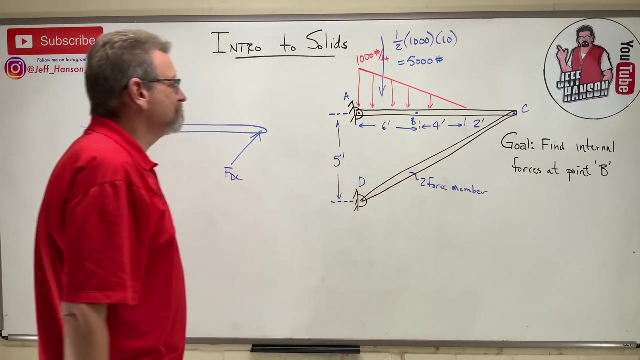 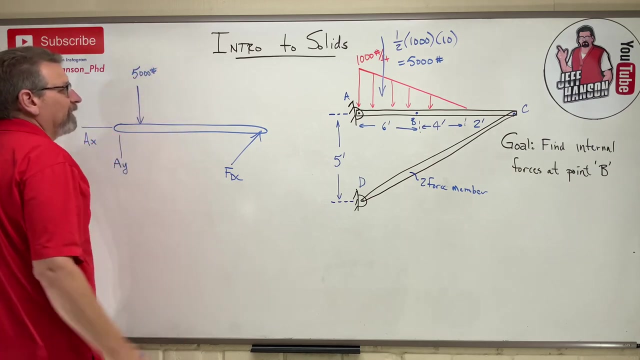 load. So we're going to turn that distributed load into a concentrated load. Do you remember how to do that? Yeah, All right. Okay, So we're going to have action. Okay, So we've been talking aboutascension previously. 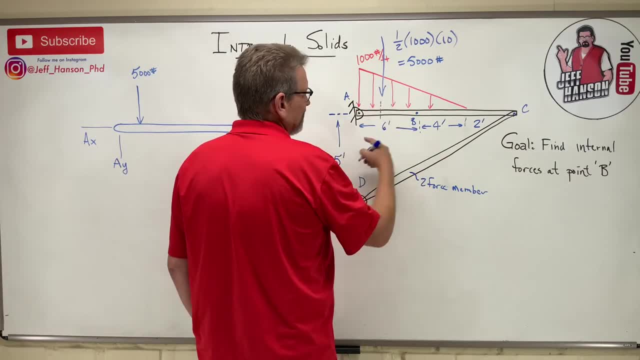 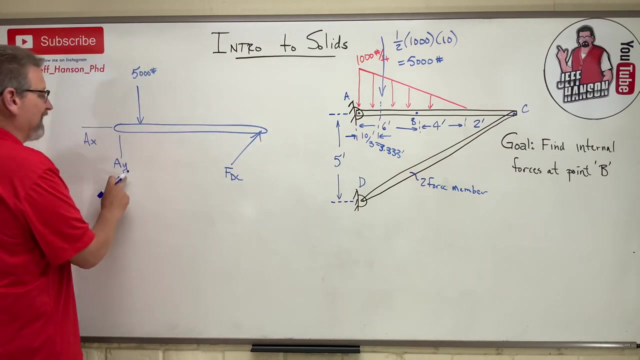 Let's try this way. Okay, Okay, All right, All right. Okay, 10 over 3, right, This little distance right here, 10 over 3 feet, right, Which is 3.33333, right? No, Yes, just 3.333 feet. okay, So let's do this. Which way does AY go? I think it goes up. 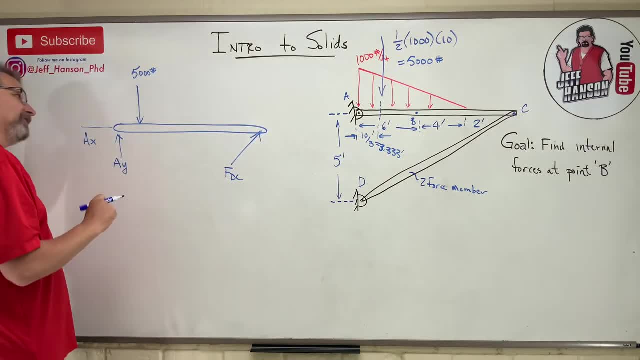 Which way does AX go? Since that guy goes to the right, I think he has to go to the left. okay, And you know, if it was up to me, I think what I'd do is take the sum of the moments at: 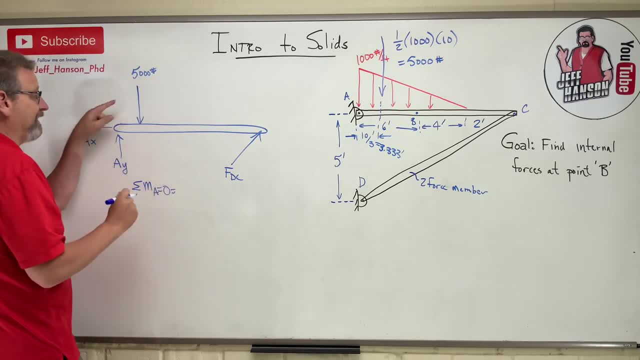 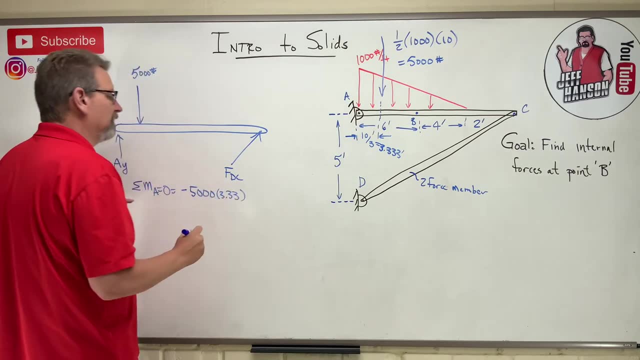 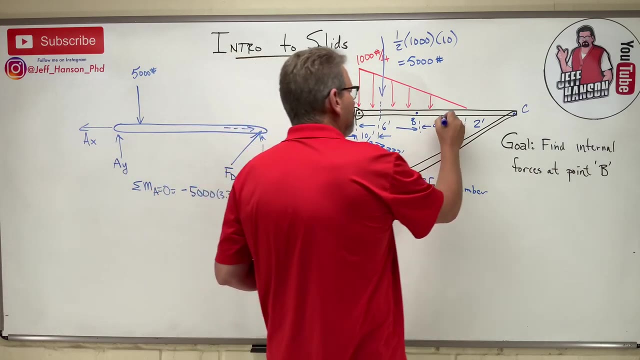 point A and I would have 5,000 rotating me negative minus 5,000 times 3.33.. And then this guy has two components over here. Oh no, we're going to have to do an angle. What is this angle? 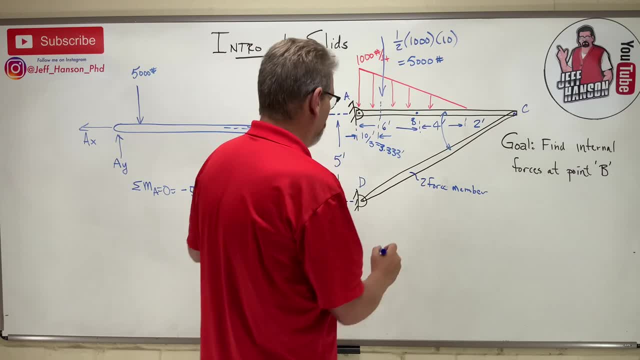 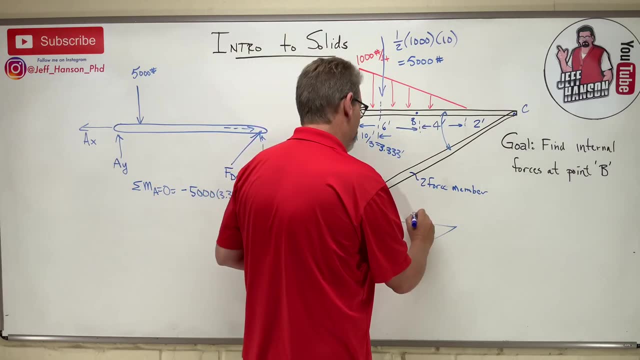 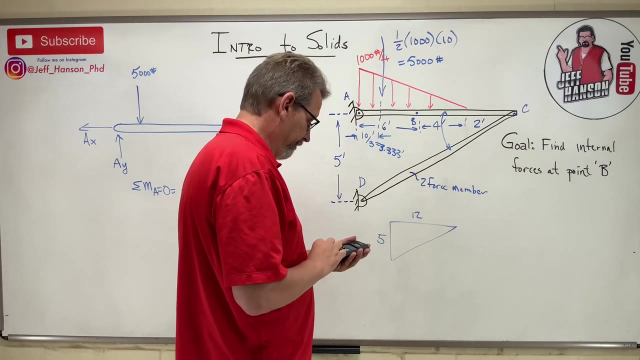 right there. Well, let's see, I got a big triangle, that's. I got a big triangle. It's got 5 on that side and it's got 10, 12 on that side. I don't know what that is, Do you? On? let's see How about tangent right? 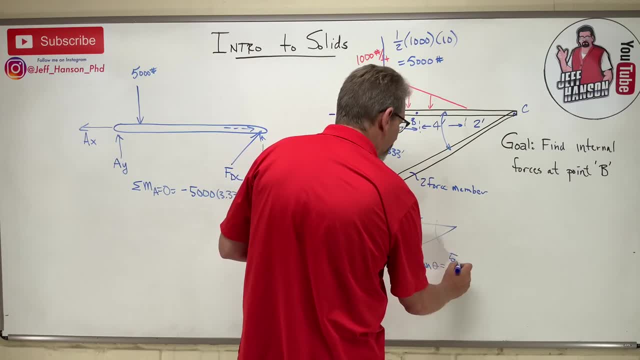 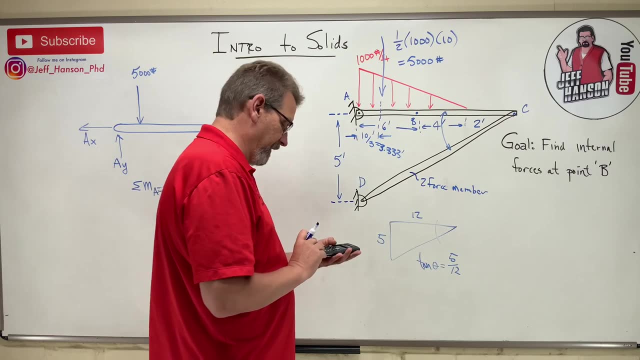 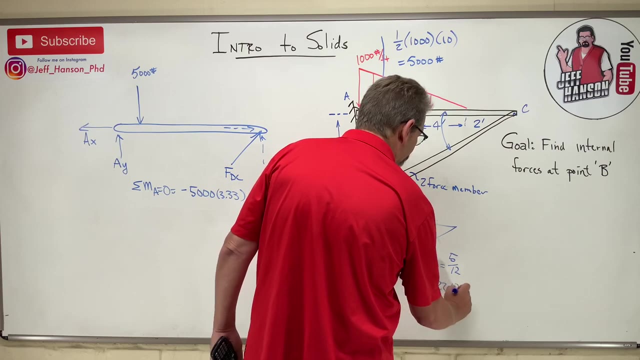 Tan theta is equal to opposite over adjacent. So 5 divided by 12 equals inverse tan of tan theta. So 5 divided by 12 equals inverse tan of tan theta. that equals twenty two point six, two, okay, twenty two point six, two degrees. so. 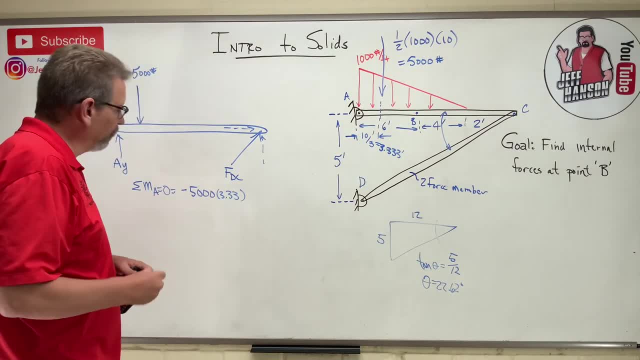 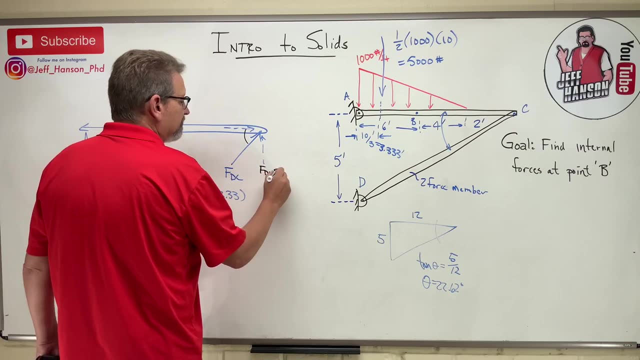 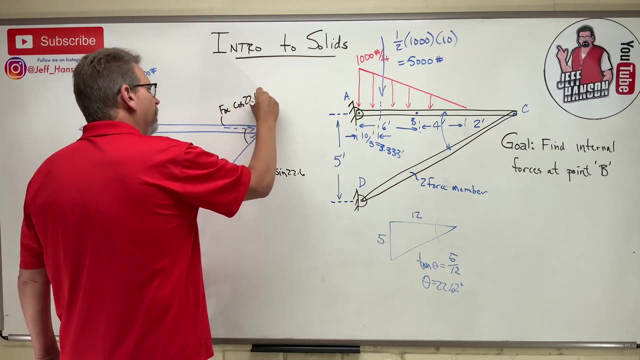 let's see, I'm changing colors. my purple is blue is not doing so good. so this is twenty two point six. so this guy over here is F DC sine twenty two point six. this guy F DC cosine, twenty two point six. okay, and this guy's a cha-cha for. 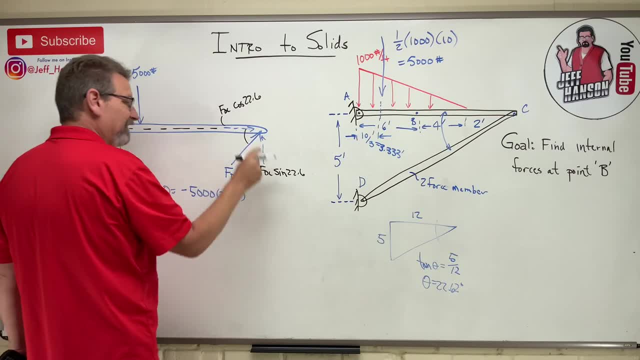 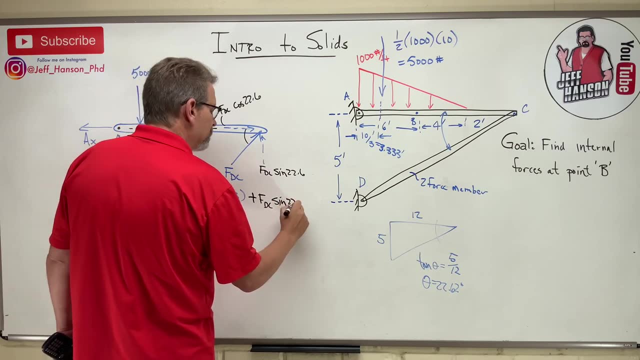 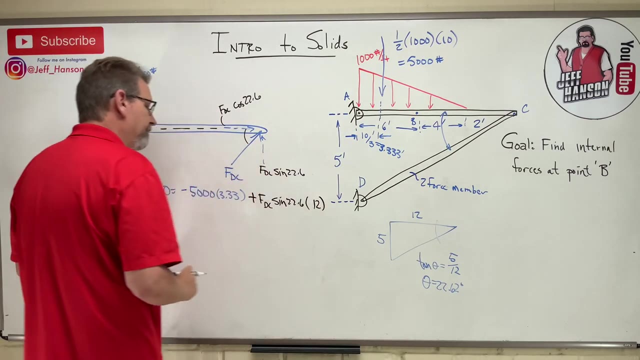 Sydney. what y'all? he goes right through point a, so he's knocked out. this one rotates me positive. so plus F, DC, sine twenty two point six times how far away. it's the whole length of beam, it's twelve. okay, so here we go, we're fixing. 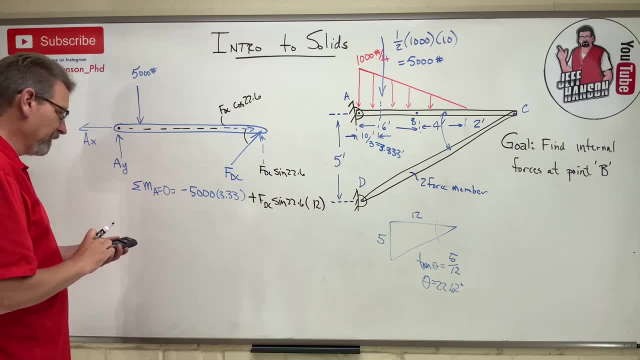 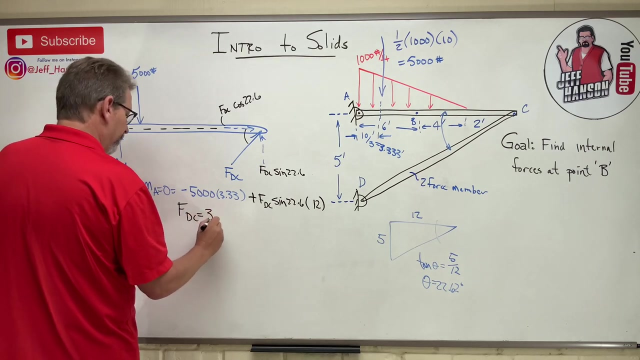 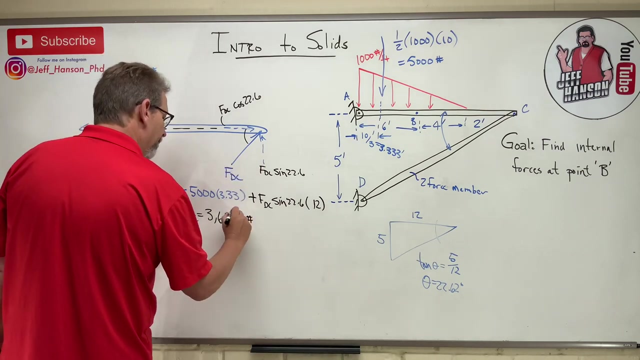 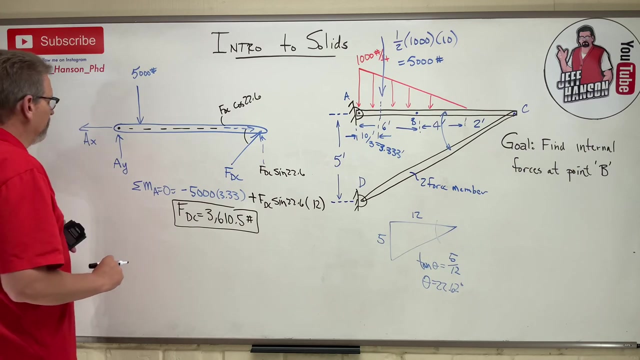 it up, DC, aren't we? five thousand times three point three, three equals divided by twelve equals divided by the sine of twenty two point six. so F? DC is equal to three thousand six hundred and ten point five pounds. two thirty-nine over 35. okayço, there's one thing that's going on, and now I can find these two guys over here. 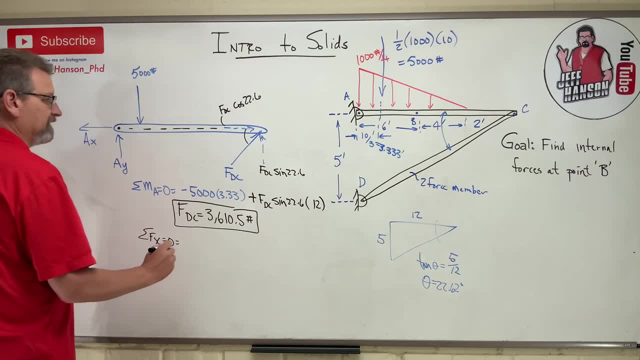 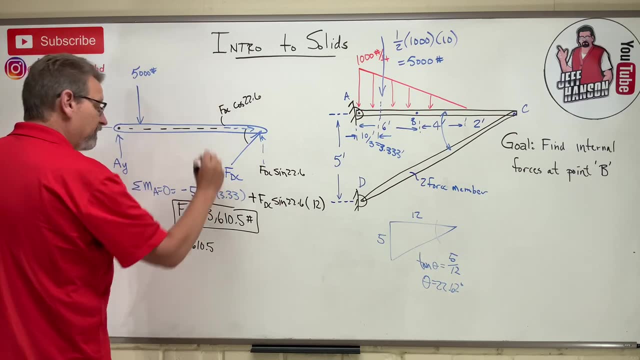 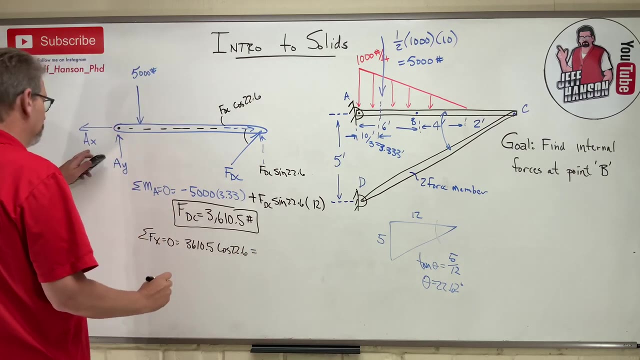 right some of the forces in the X, and so I get 36, ten point five right times. the cosine twenty two point six is equal to unbox is equal to 3610.5. cosine of 22.6 equals 33, 33.25. 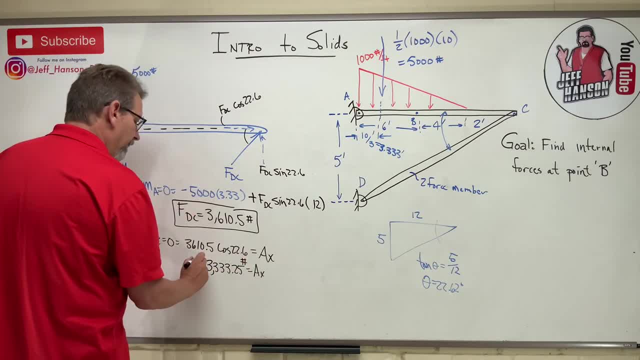 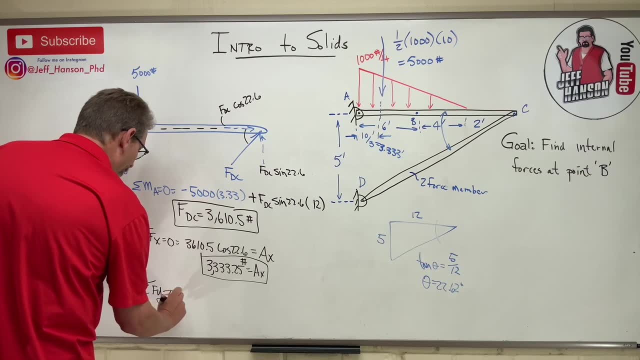 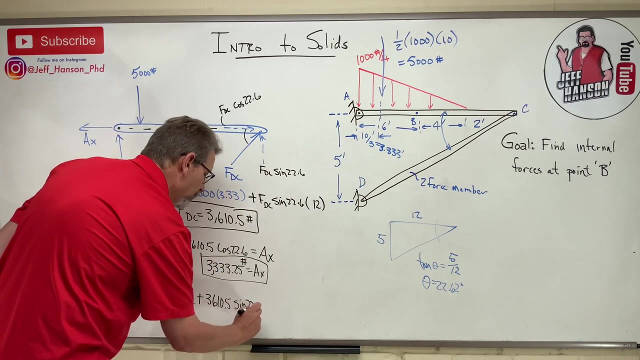 that's pounds, okay. and then of course, a y. pretty easy to find a y, sum of the force and the y, and in the y i've got a y, i got that guy plus 36, 10.5, sine 22.6, and then i got this guy. 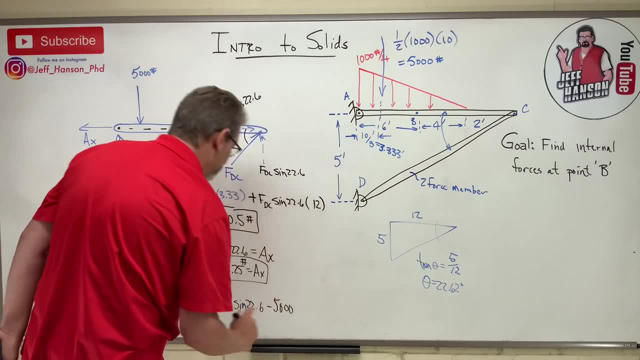 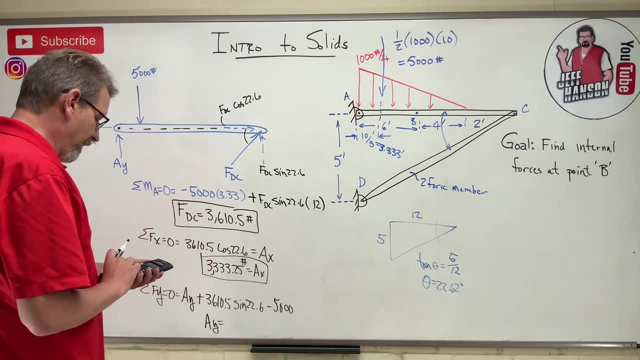 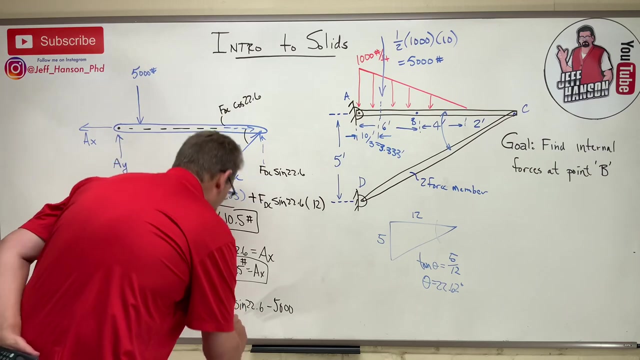 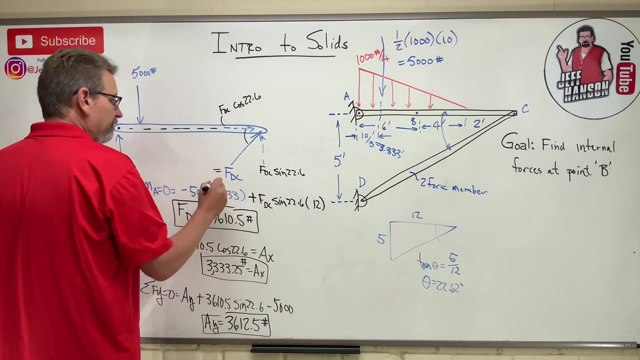 minus 5000. so a y is equal to 5000 minus 36, 10.5 times the sine of 22.6, 3612.5. so there's the first bit of stuff that i need: right fdc um 36, 10.5. 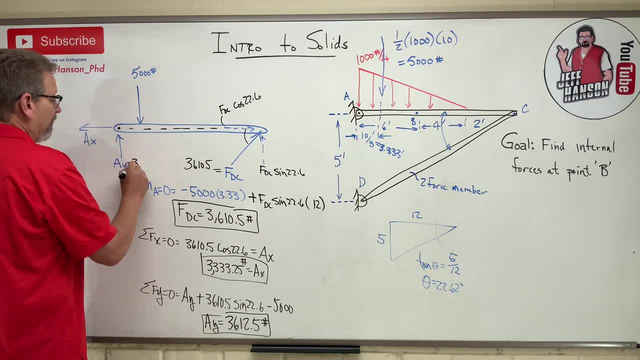 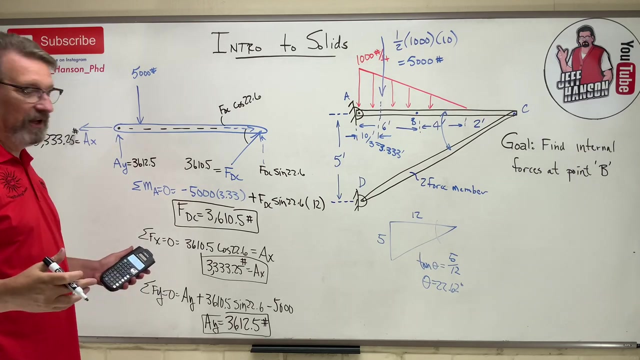 five a y, 36 twelve. point five a x a x. where'd you go ax? there he is 33, 33.25. okay, So there's step one. I got global equilibrium. What's the next? Is there more? Yeah, we haven't. 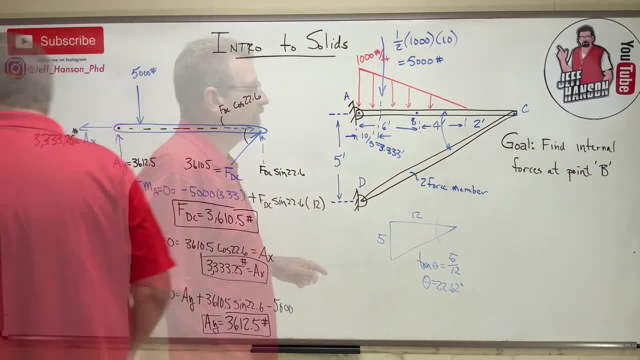 even found out what's going on point B. yet Let me erase this. Let's do that, All right. So how do I find out what's going on? point B? Remember, we cut it right. We cut the beam. 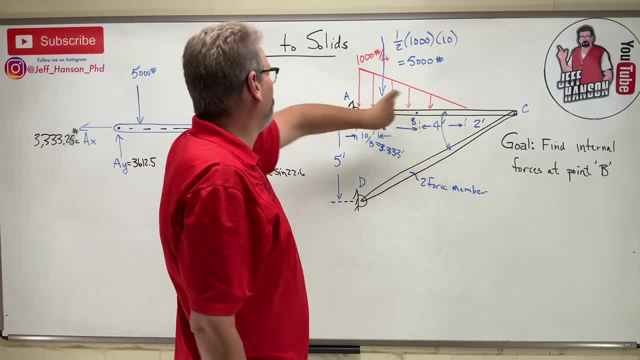 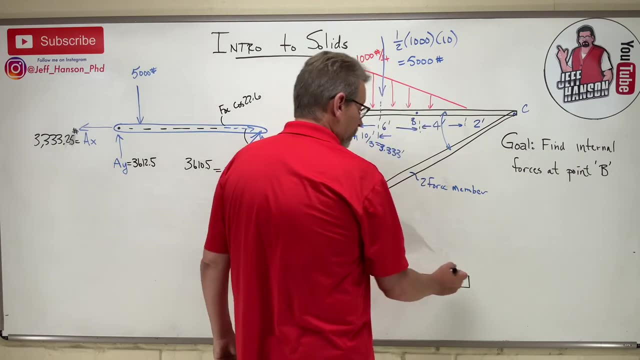 You can draw the right side or you can draw the left side. I think I'm just going to draw the left side, So here I go. Here's the beam. Okay, What's on that beam? Well, there's a distributed load that kind of looks like that. 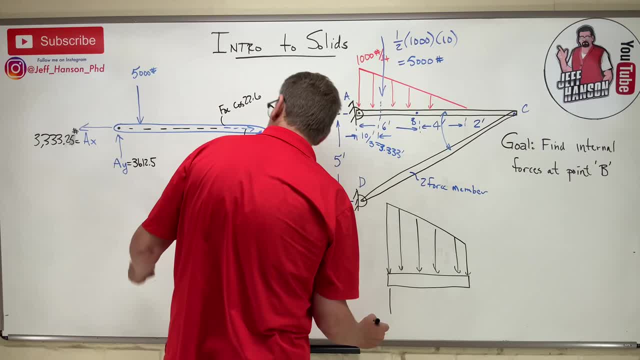 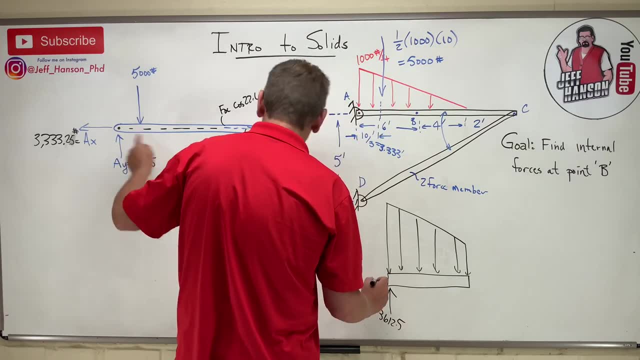 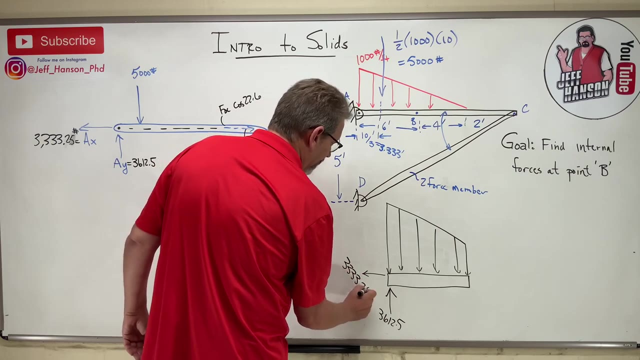 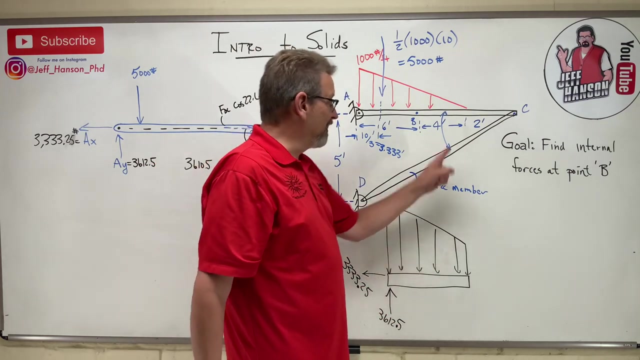 And then over here at A, I've got this right, I've got 3612.5.. And I've got this guy which is 3333.25.. And then, what else do I have? Well, what happens when you cut a beam, Do you remember? Of course you do. You must have an M and 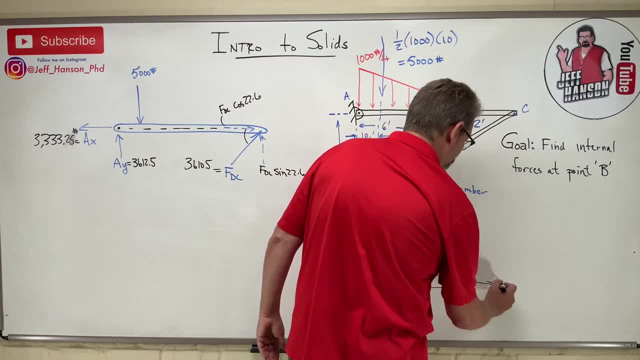 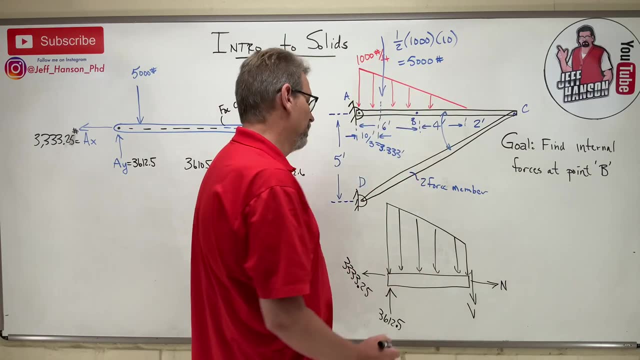 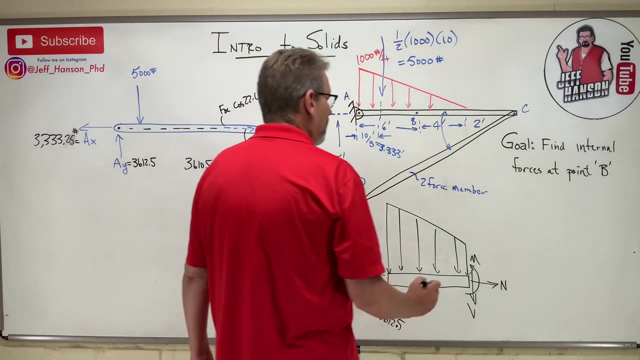 V right. Here's your N. Here's your V. We drew the left side. You don't want to get left at Walmart or you'll feel down. And then here's your M. Remember that's from our positive sign convention. Okay, Now at point B. 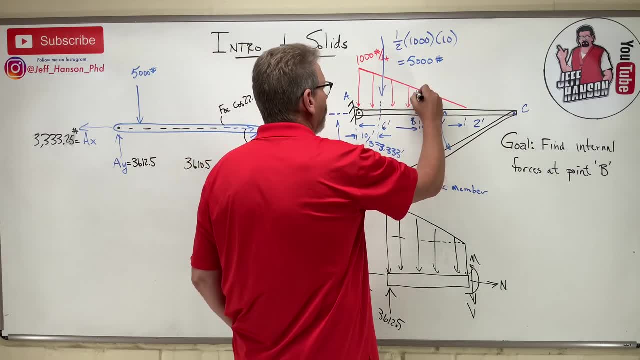 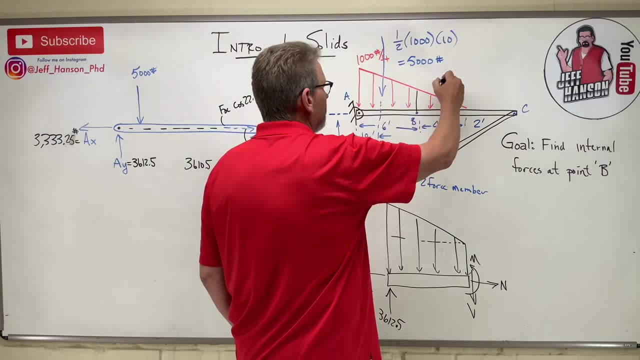 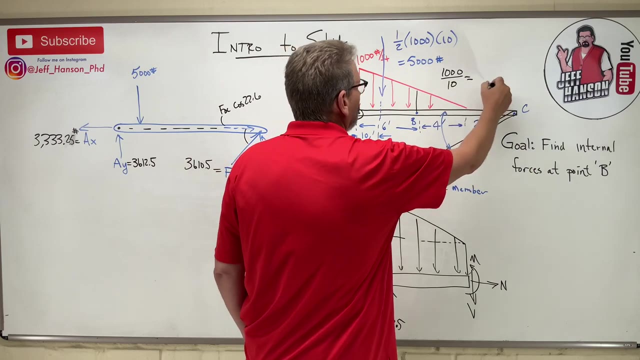 do we know how tall this curve is at point B? Well, yes, we can do similar triangles and figure that out, can't we? So over here, we say 1,000 is to 10, as 4 is to, we'll call it Y. That's how. 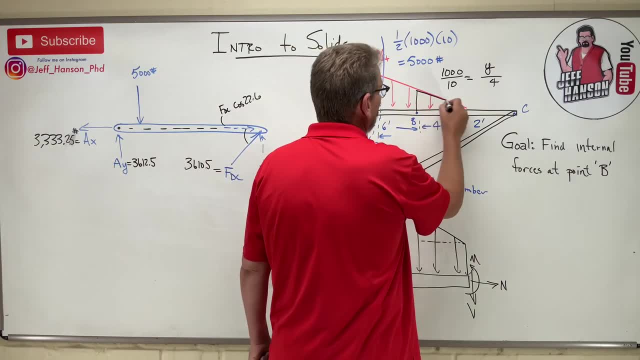 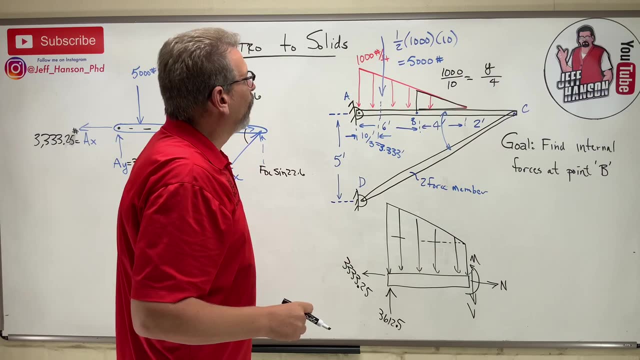 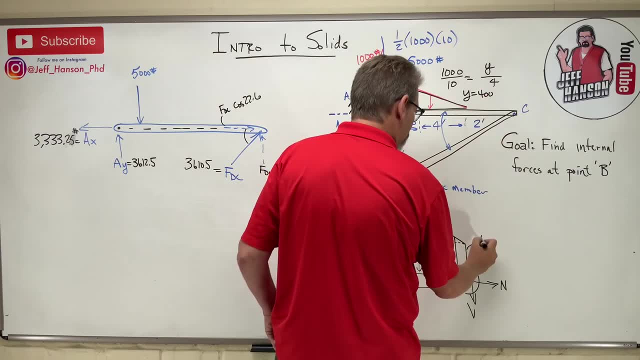 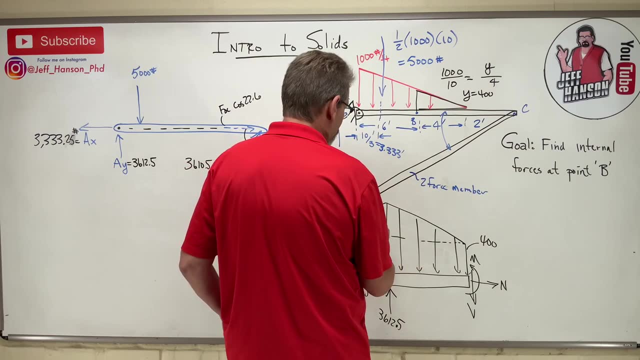 equals 400. So this height right here is 400, which means that this height over here has to be 600, because it's 1,000 on that end over there right, And we know this distance here is 6,. 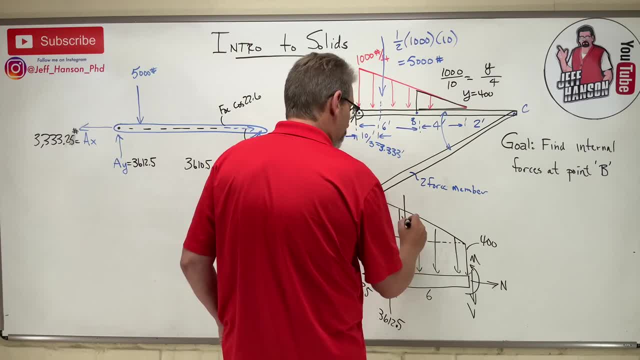 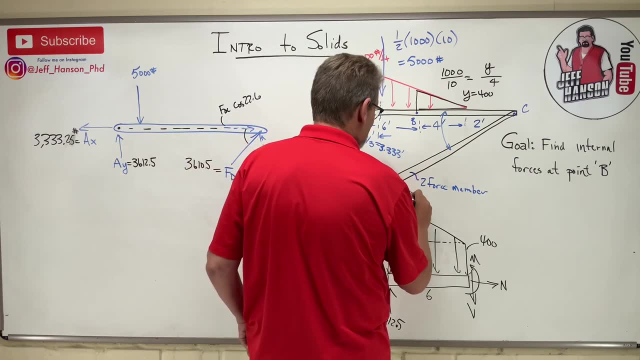 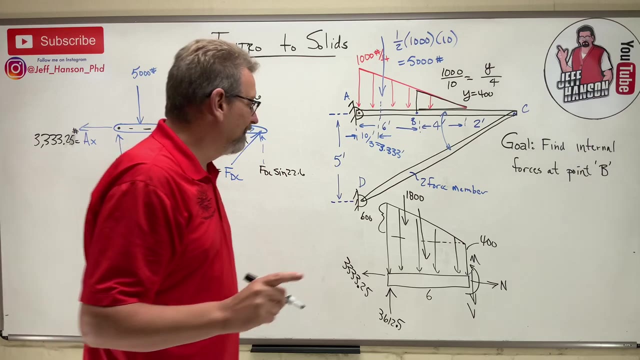 right, So just the triangle part is going to be 1 half base times height. 6 times 6, is 3,600. divided by 2 is 1,800.. And the rectangle part down here is 400 tall by 6 wide. That's going. 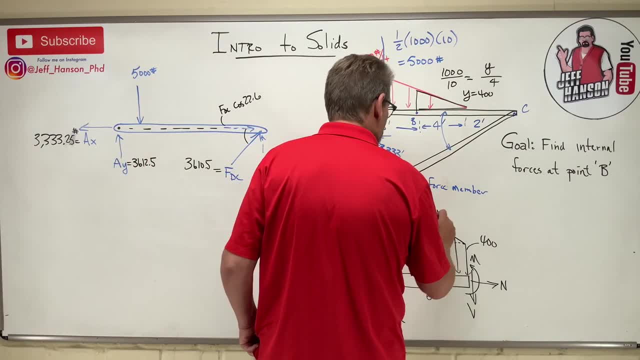 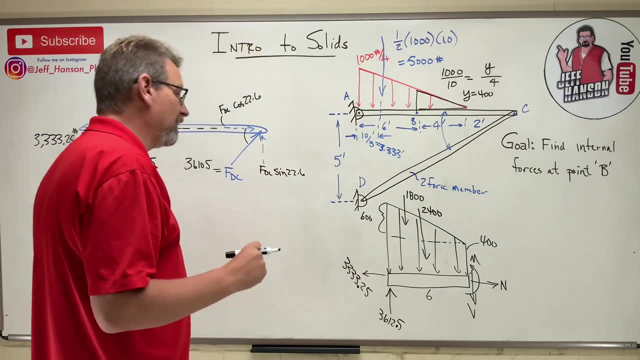 to be 2,400.. So I'm going to treat it as like two concentrated loads there, right? Because it's a triangle stacked on top of a rectangle. Okay, All right, Let's find the things right. This is going. 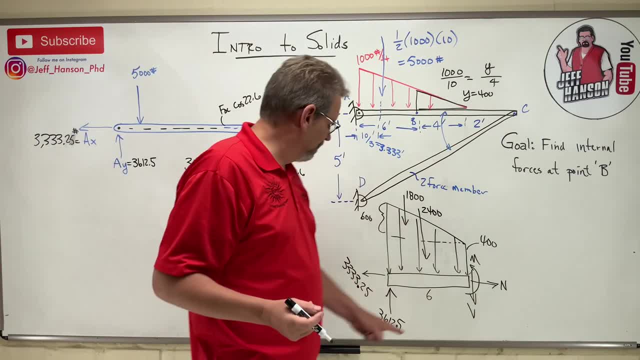 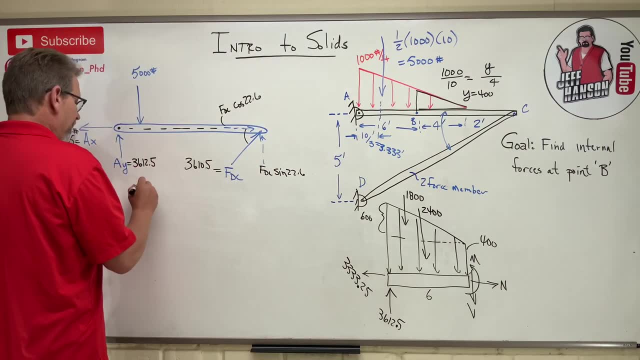 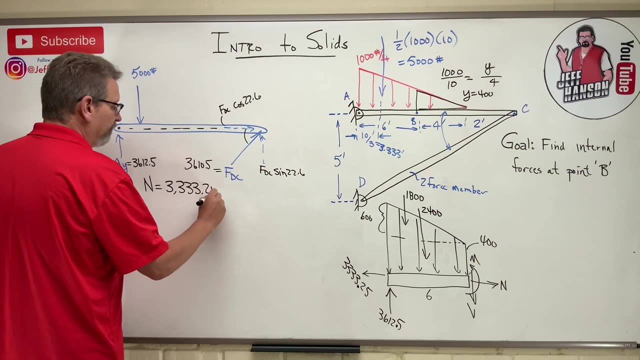 to be pretty easy. How big is the end going to be? Well, how much other stuff do you see in the X direction? Because I only see one, So right away. N is equal to 3,333.25 pounds. There's one. 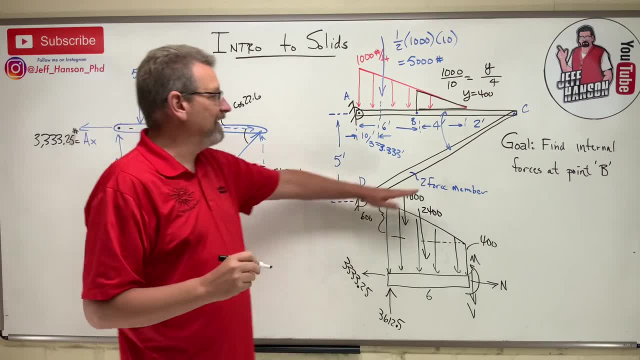 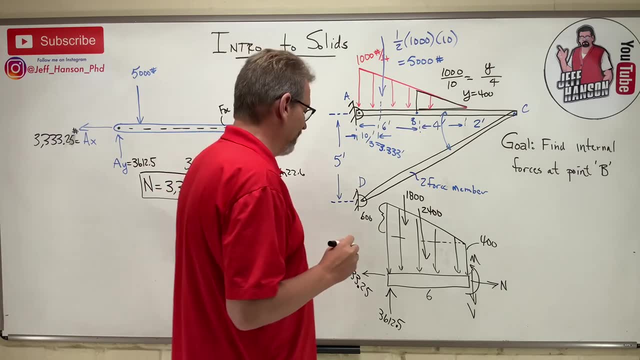 of the three things that we have to find. We're trying to find the internal force. at point B, Number two, how do we find V? Well, how about some of the forces in the Y? So what do we get? We get some of the forces in the Y. 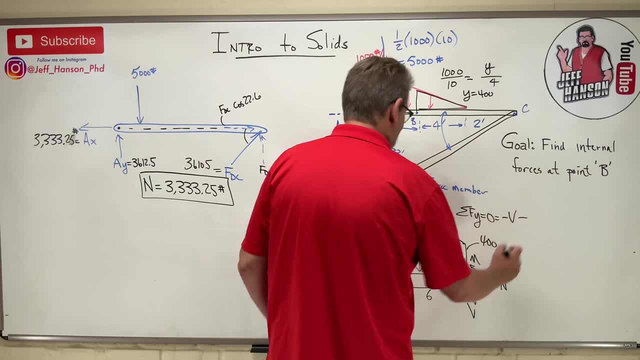 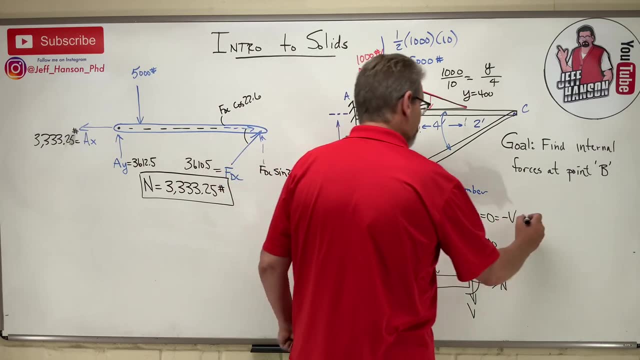 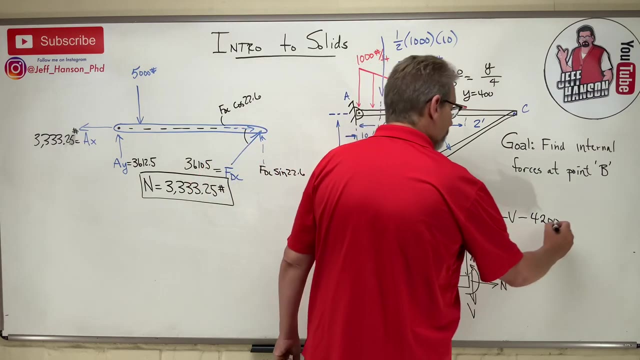 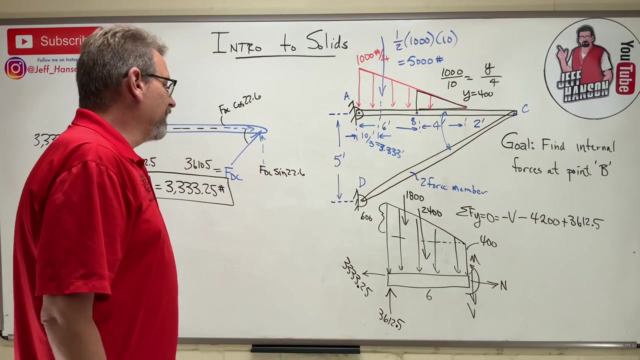 equals negative V minus 1,800, plus 2,400.. That's what? 3,400, 4,200.. And then plus 3,612.5.. Okay, So we're going to get a negative number for V, aren't we? Yes, we are. 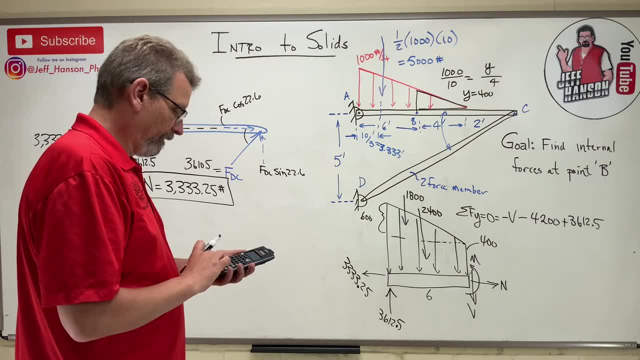 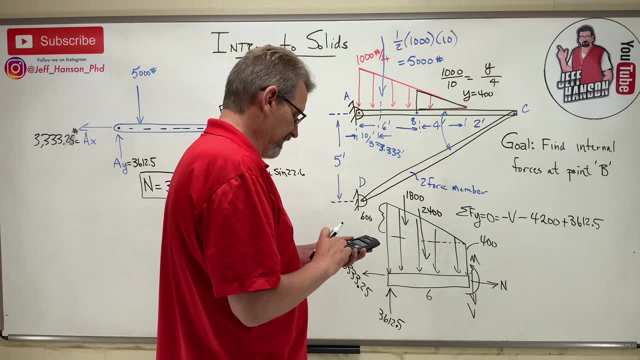 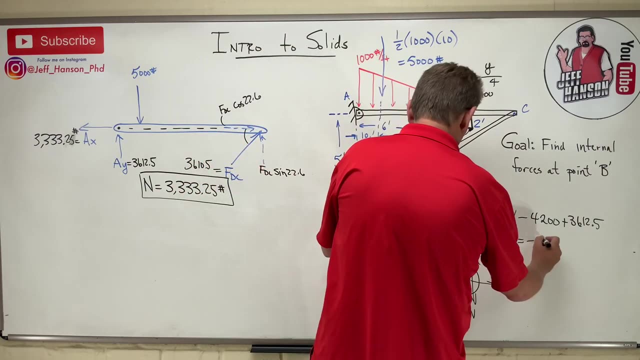 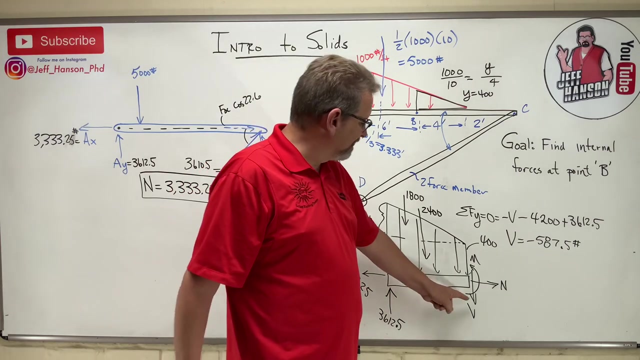 All right, And so what do we get? We get 4,200 minus 3,612.5.. So we're going to get: V is equal to negative 587.5 pounds. Okay, Well, what does that mean? Well, it just means that. 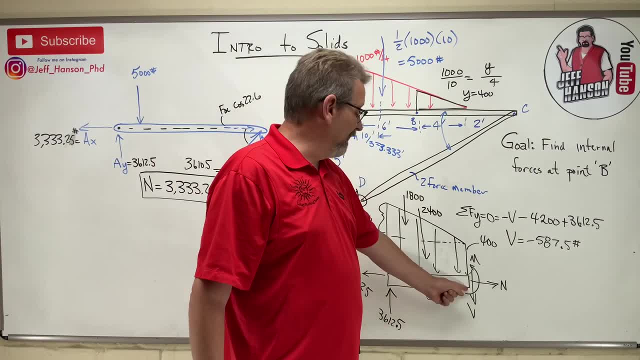 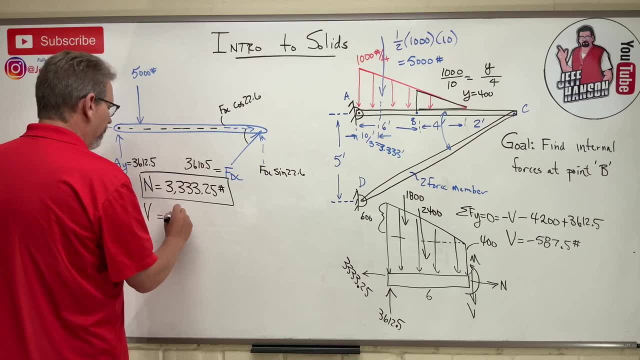 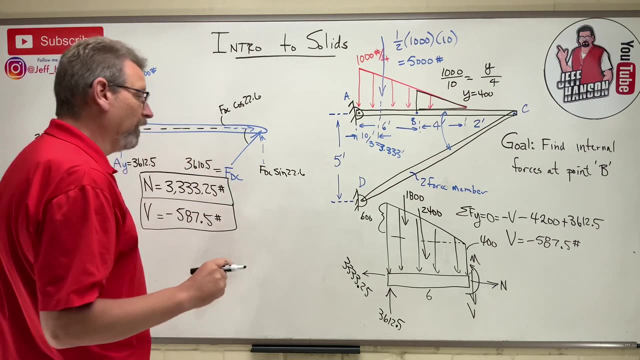 the positive sign convention said V should go down, but really V on this side of the free body should go up, So that's no big deal. So V negative 587.5 pounds And one more. that is what is M. Well, we can get that guy by taking the sum of the moments. 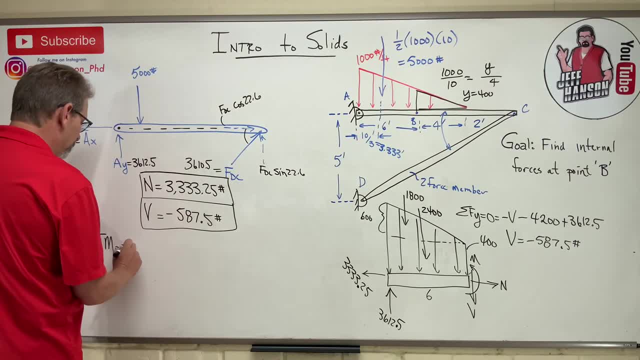 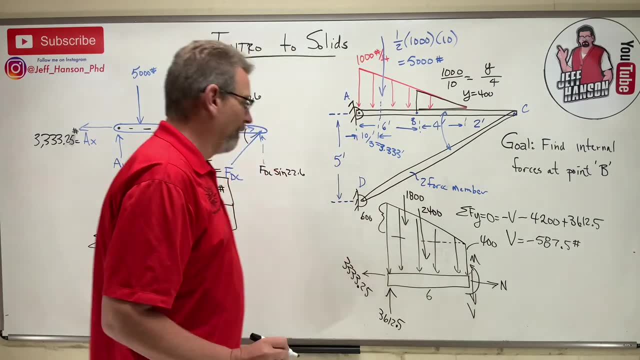 I'm going to take the sum of the moments at point B, where we cut it, And what do we get? We take the sum of the moments here. We knock out N and V, but you can't knock out a moment. So that's going to be a positive M. 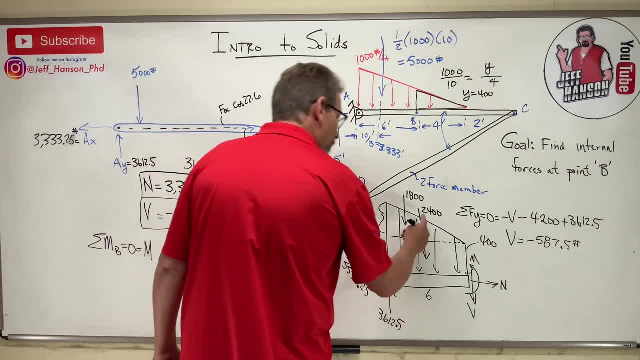 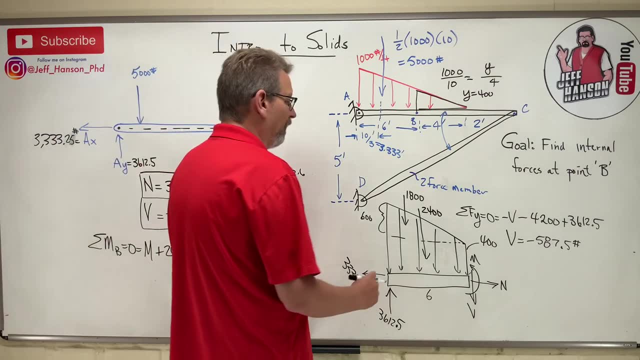 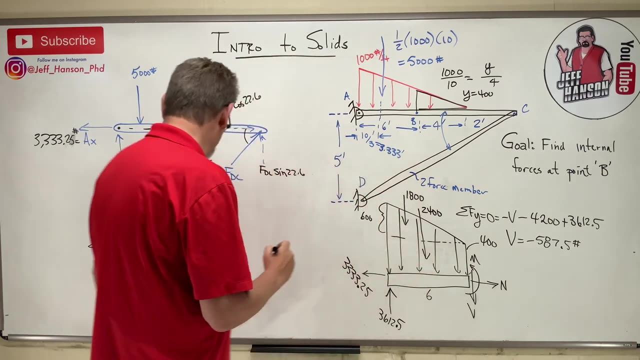 It was a positive moment. The 2,400 rotates me positive. So plus 2,400 times, how far away, Well, from the cut which is here to where that moment is, which is half of six, it's three. 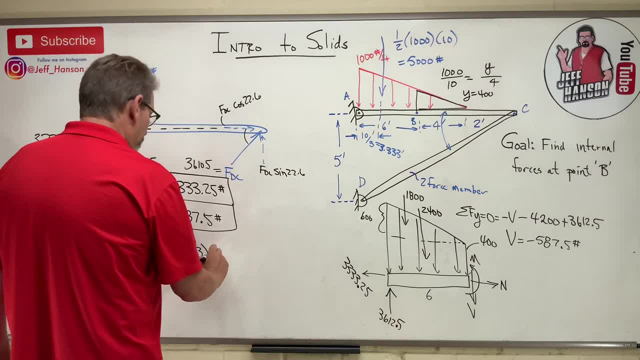 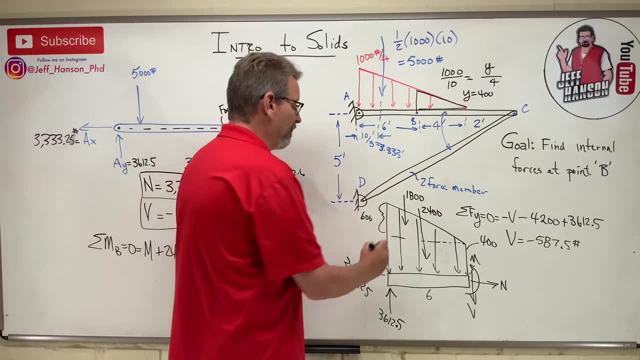 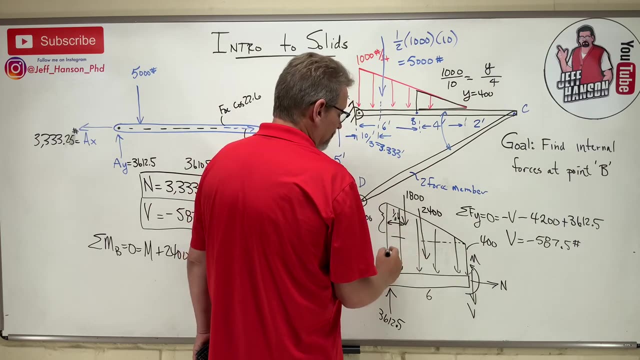 isn't it Okay, Plus 1,800 times. how far away is that guy? Well, remember, it's a centroid of a triangle. So this is. So if the whole thing is six, then this must be What's the third of six. Two right Two. 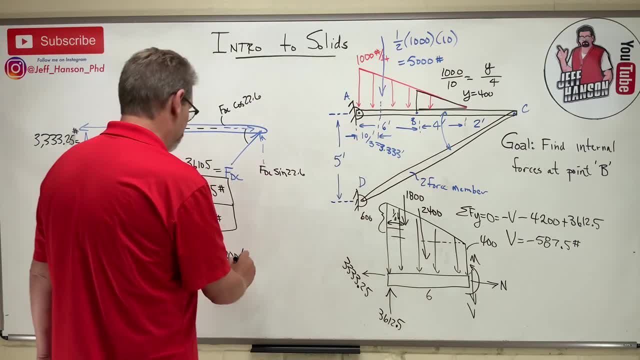 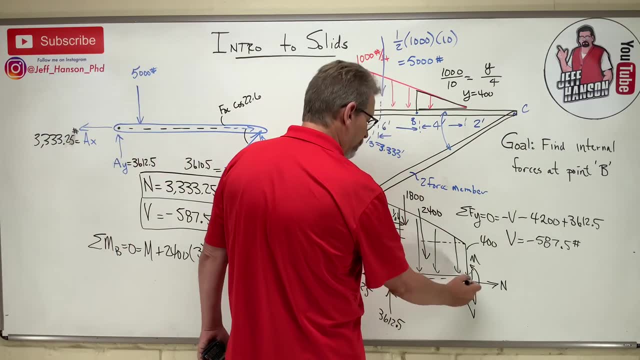 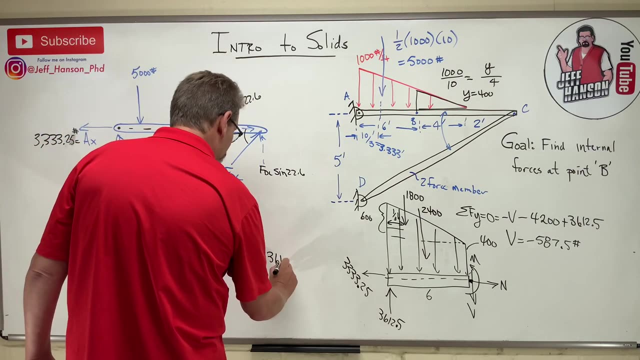 over here, which is four from that end over there, isn't it Four? And then the 3,333, he gets knocked out. He goes through this point B over there And then the 3,612 rotates me negative Minus 3,612.5 times. how far away. 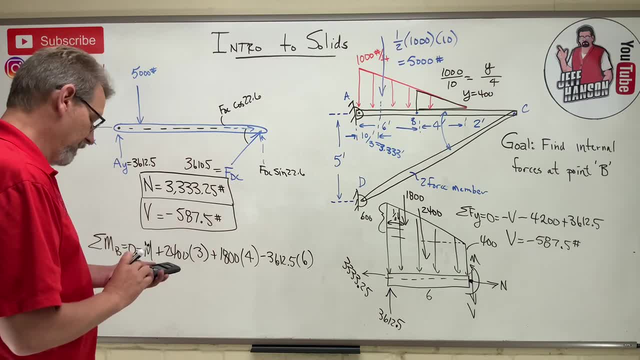 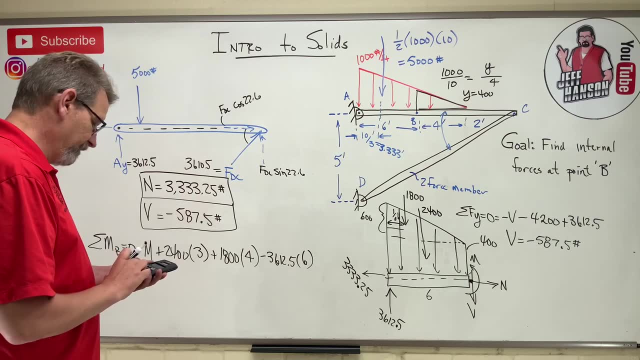 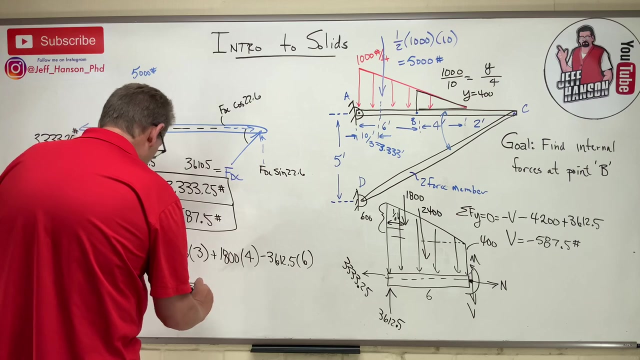 Six. Okay, So here we go. So 3,612.5 times six minus 1,800 times four minus 2,400 times three equals 7,275.. The moment at point B is equal to 7,275. what?